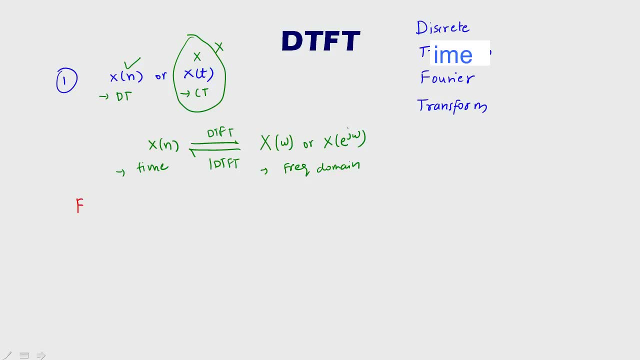 that what we are doing, but how we can convert. Now comes the formula. So what is the formula? to convert one signal from time domain to frequency domain using DTFT, Because DTFT and DFT are two separate terms, two separate concepts. 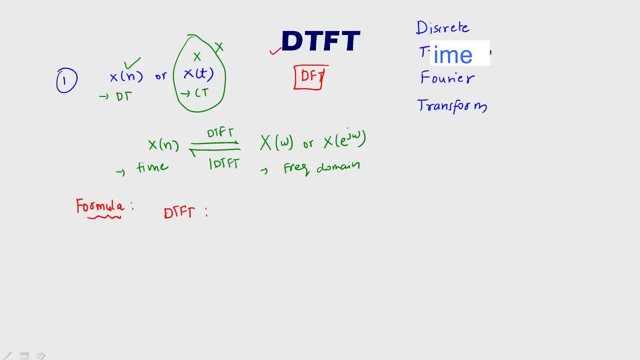 So that's why for DTFT, the formula is: we have. if we are converting x of n to x of omega, we are using DTFT. So the formula is: we need x of omega, So x of omega is equal to summation of n is equal. 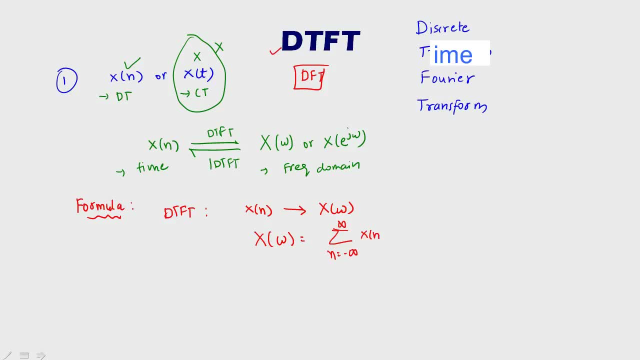 to minus infinity to infinity. then x of n e raised to minus j omega n. Now this is similar to Z transformation, correct? So if you have studied the Z transformation, if you haven't, please do watch my previous videos on Z transformation. you will get. 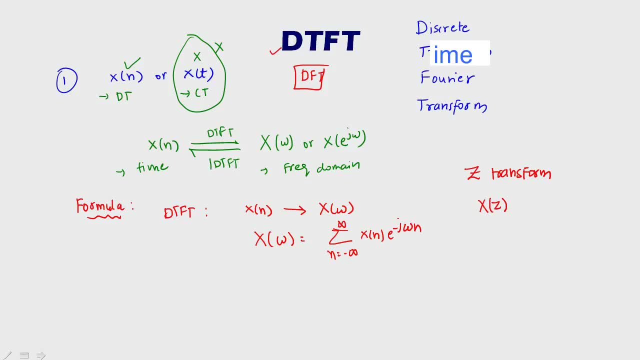 the idea. In Z transformation we need x of z. then we use the formula: summation of n is equal to minus infinity to infinity, x of n, z raised to minus n. So you can see the similarity between Z transformation and DTFT. Tell me the similarity. Similarity is: if you put z is equal to 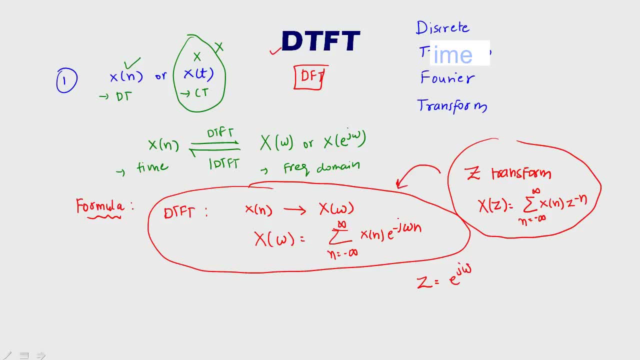 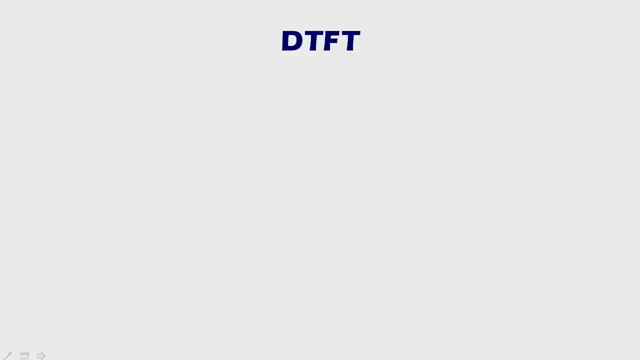 e raised to j omega, you will get DTFT, and that's why it is said that if you know Z transformation, DTFT is a cakewalk for you. Now what if I say I have x of omega and I need x of n? that is, I have a signal. 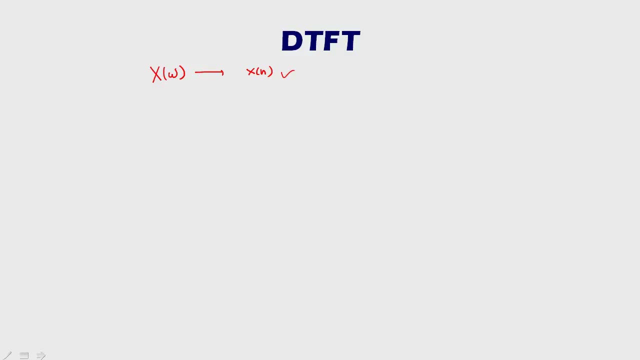 in frequency domain, but now I need a signal in time domain. then you have to use inverse discrete time, Fourier transform. So now comes the IDTFT formula. So now, what is the formula for that? x of n is equal to 1 by 2 pi. 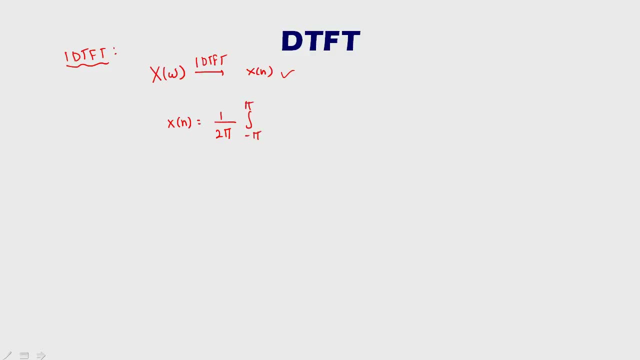 then you have integral of minus pi to pi and then you have x of omega, correct. then it is multiplied with e raised to j omega and D omega. So this is the formula if you have this x of omega and you need x of n. So this is: 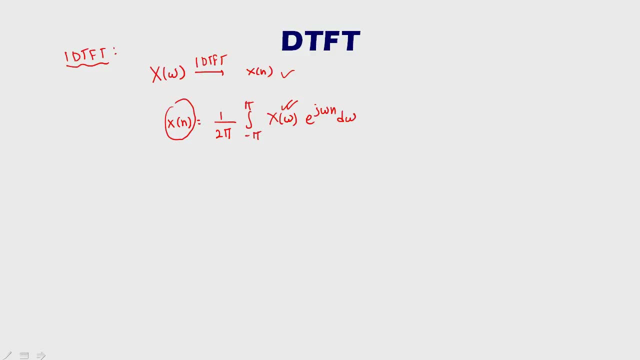 IDTFT. Now comes the important part: what we are trying to do. What we are trying to do Why we are studying this topic. So let's see that answer as well. So, basically, we do DTFT to find the magnitude. 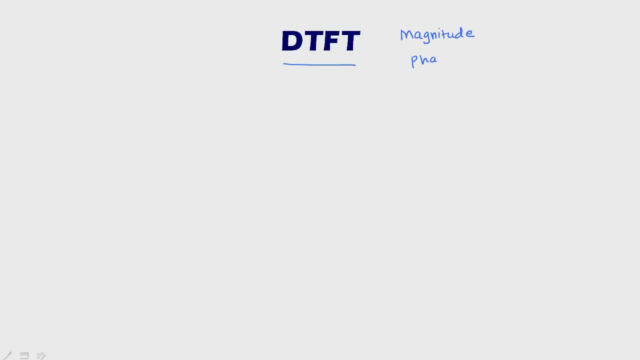 and we are trying to find the phase of a signal because we have x of omega. So let's look at this concept as well. Your x of omega can be of two types. One, it can be polar form or it can be in rectangular. 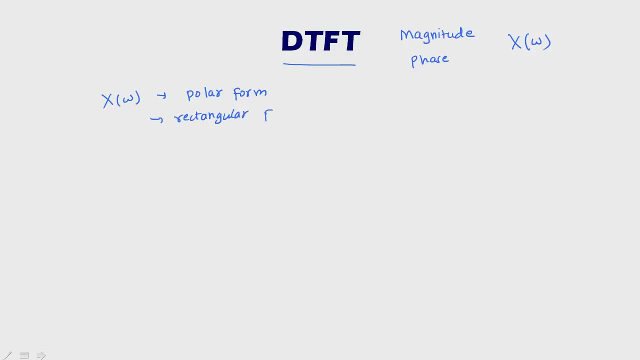 form. Now, if my signal is in polar form- so this is the first point- let me take that If my signal is in polar form, I have to take a special care, because x of omega is equal to mod of x of omega into angle of x of. 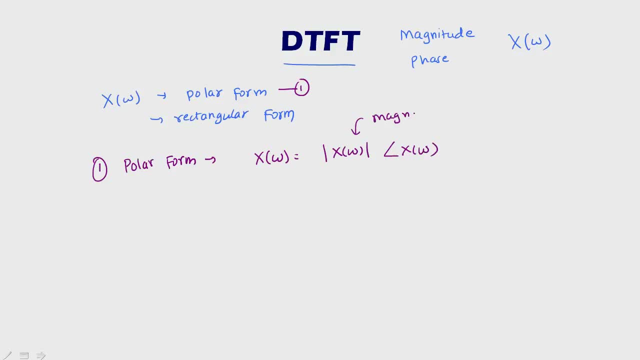 omega. So from here I will get the magnitude and from here I will get the phase. But now if my signal is in rectangular form, so rect form, then we have some additional step, because now my x of omega is in the form of. we have the real part, so xr of 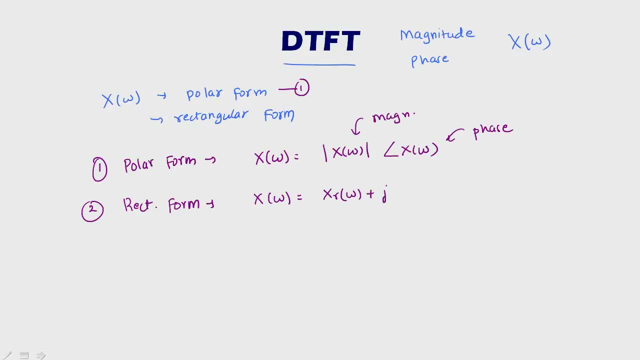 r means the real xr of omega plus j times xi of omega. So this is similar to a plus ib. So this is the real part, This is the imaginary part, So this is the form From this we have to find. 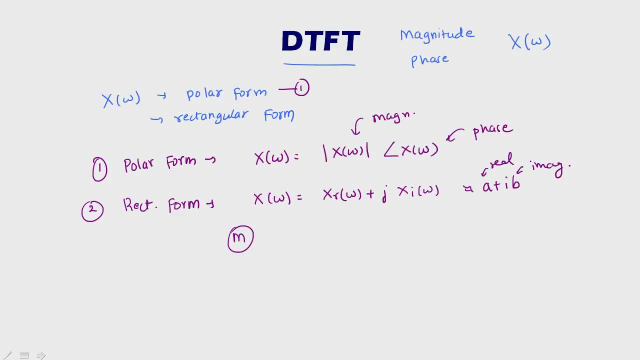 the magnitude and phase. So you have to find the magnitude, What you have to do. So, mod of x, of omega, you need that is equal to root of real part, square, So square of the real part plus square of the imaginary part. And also, if you need the 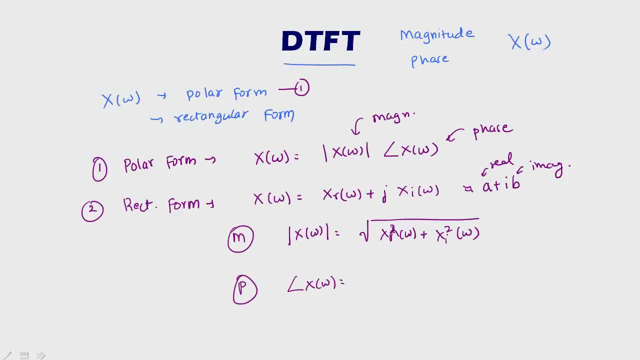 phase, the formula goes in a different fashion. So angle is equal to tan inverse of real part. Okay, imaginary part is in the numerator and upon the real part. So this is the formula and these are the two types. Very important concept because 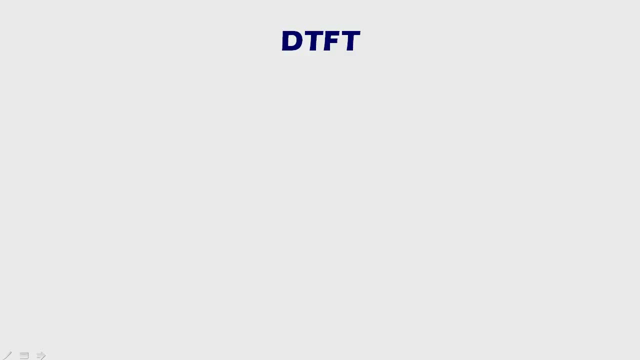 we do DTFT to find the magnitude and phase. So when we talk about the application of DTFT, there are many applications possible. One is I have studied personally is about the speech processing. So this is the PhD subject and a very important subject for MTech students as well. 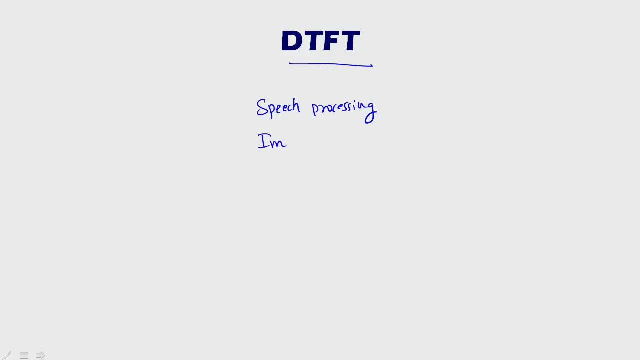 Speech processing and it is also present in image processing, So you can find various application. in signal processing You have various applications, So it is very important to find DTFT because we can apply this concept in every subject possible: Speech processing, image processing.